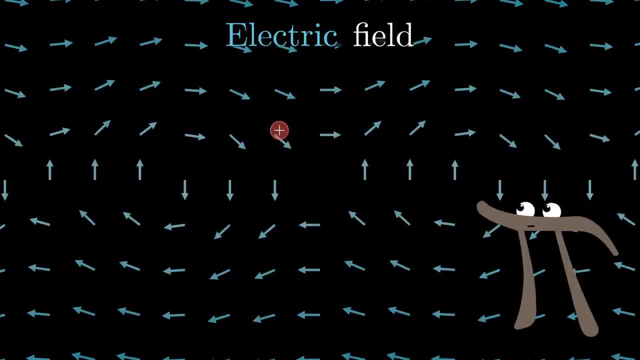 of the field. Now, the physical meaning of those arrows is that if you have some charged particle in space, there's going to be a force on that particle in the direction of the arrow and it's proportional to the length of the arrow and the specific charge of the particle. 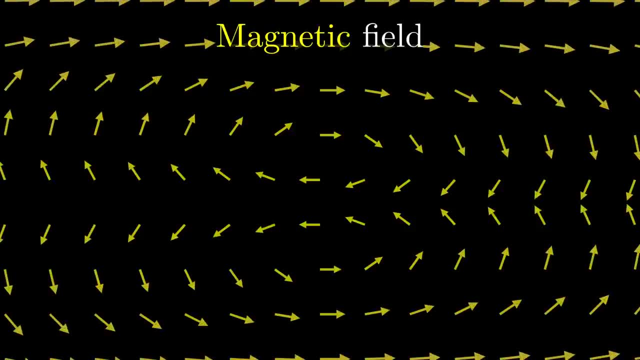 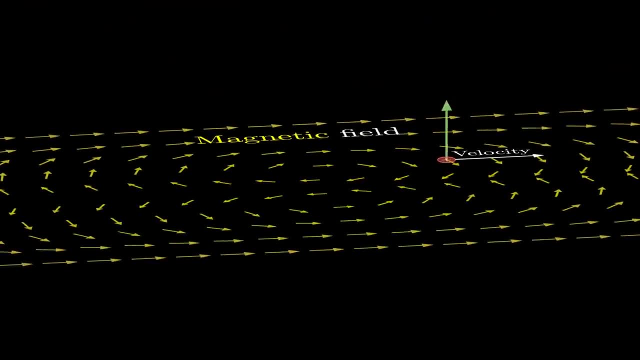 Likewise, the magnetic field is another vector field where now the physical meaning of each arrow is that when a charged particle is moving through that space, there's going to be a force perpendicular to both its direction of motion and to the direction of the magnetic field. 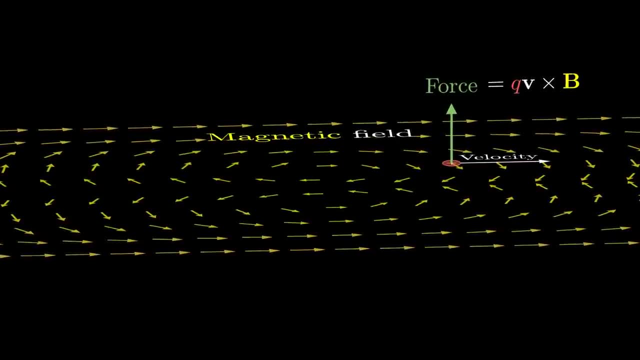 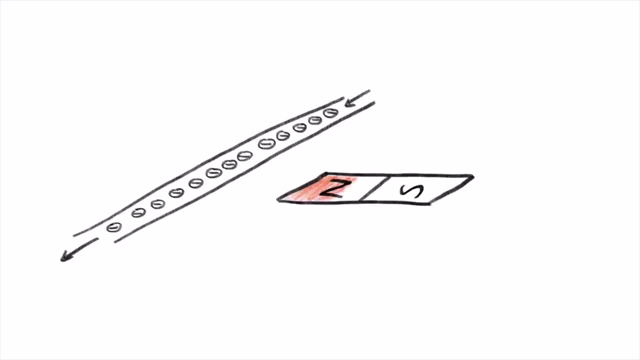 and the strength of that force is proportional to the charge of the particle, its velocity and the length of the magnetic field arrow. For example, a wire with a current of moving charges next to a magnet is either pushed or pulled by that magnetic field. A kind of culmination of the 19th century physics understanding. 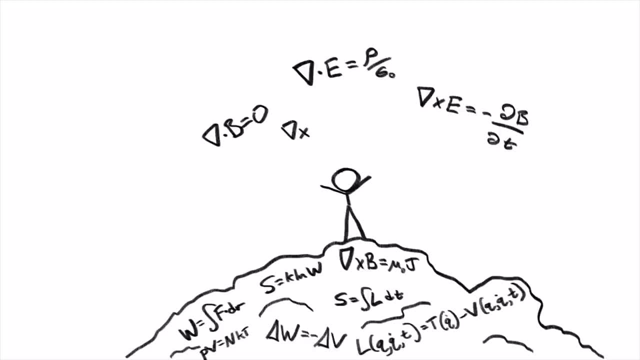 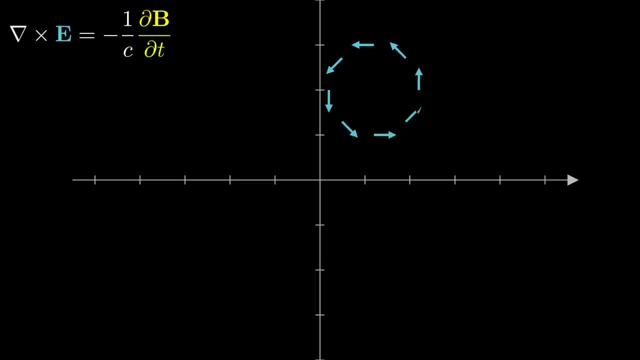 of how these two fields work are Maxwell's equations, which, among other things, describe how each of these fields can cause a change to the other. Specifically, what Maxwell's equations tell us is that when the electric field arrows seem to be forming a loop around some region, the magnetic field will be increasing inside. 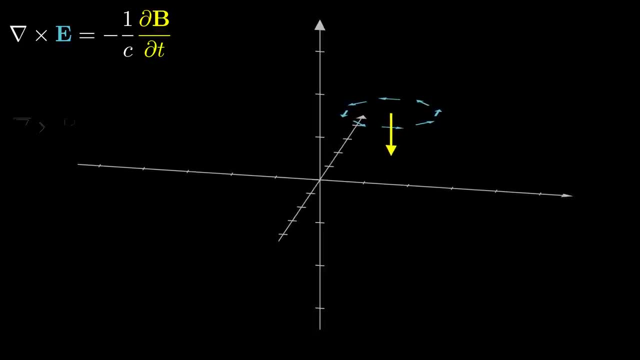 that region perpendicular to the plane of the loop And, symmetrically, such a loop in the magnetic field corresponds to a change in the electric field within it perpendicular to the plane of the loop. The specifics for how exactly these equations work is really beautiful and worth a full. 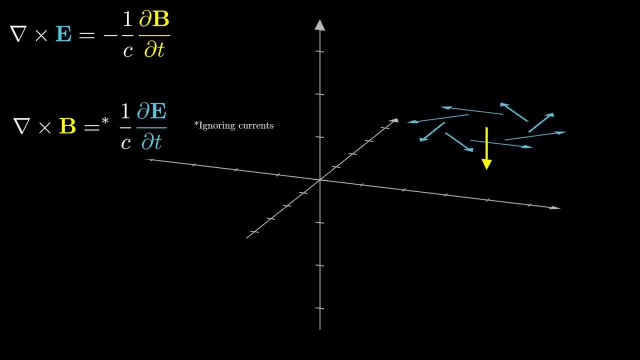 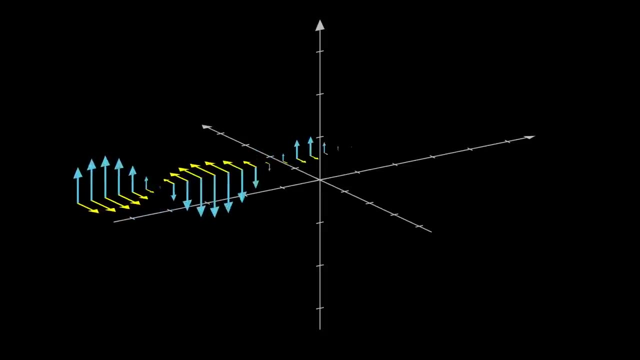 video on its own. but all you need to know for now is that one natural consequence of this mutual interplay in how changes to one field cause changes to the other in its neighboring regions is that you get these propagating waves where the electric field and magnetic field 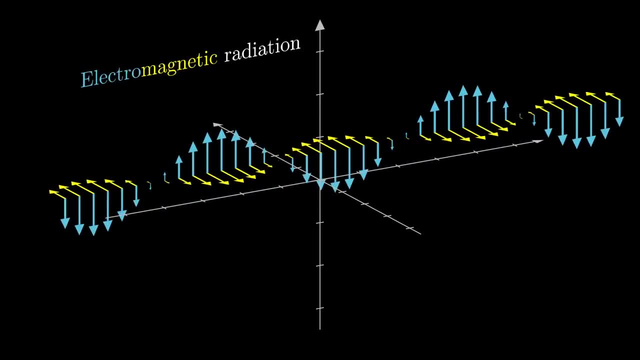 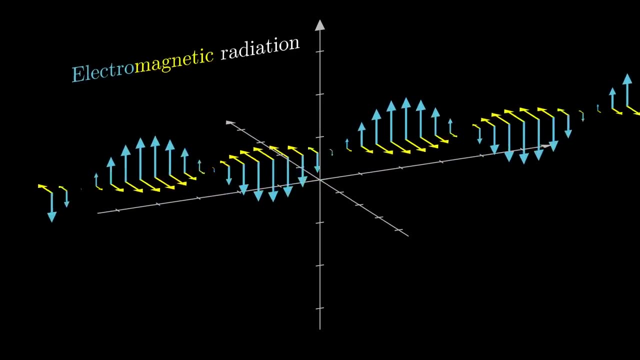 are oscillating perpendicular to each other and perpendicular to the direction of propagation. When you hear the term electromagnetic radiation, which refers to things like radio waves and visible light, this is what it's talking about: propagating waves in both the electric 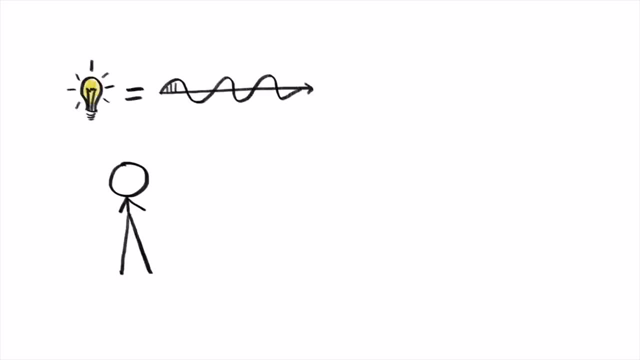 and magnetic fields. Of course it's now almost mainstream to know of light as electromagnetic radiation, but it's neat to think about just how surprising this was in Maxwell's time, that these fields that have to do with forces on charged particles and magnetic fields are actually propagating. 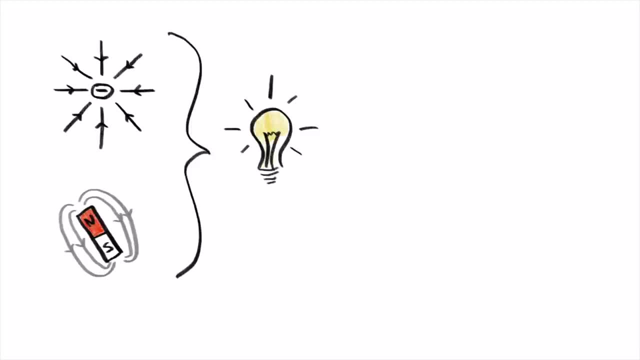 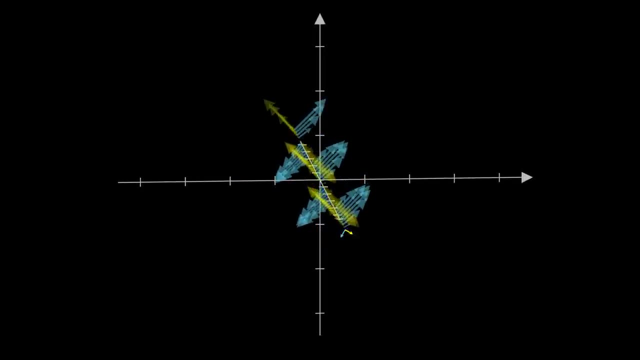 It's not only about light, but that what light is is a propagating wave, as these two fields dance with each other, causing this mutual oscillation of increasing and decreasing field strength. With this as a visual, let's take a moment to lay down the math used to describe waves. 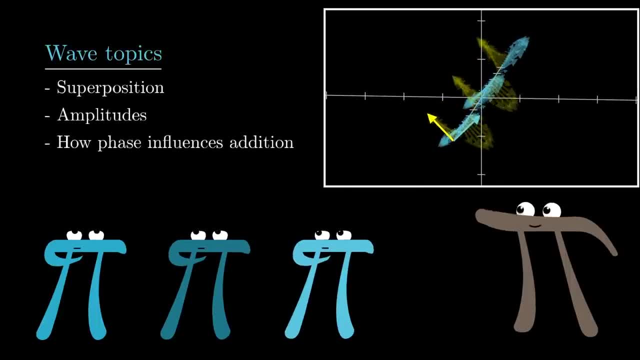 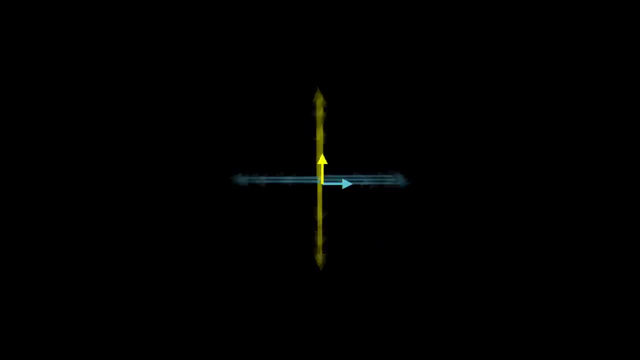 It'll still be purely classical, but ideas that are core to quantum mechanics, like superposition, amplitudes, phases, all of these come up in this context and, I would argue, with a clearer motivation for what they actually mean. Take this wave and think of it as directed straight out of the screen towards your face. 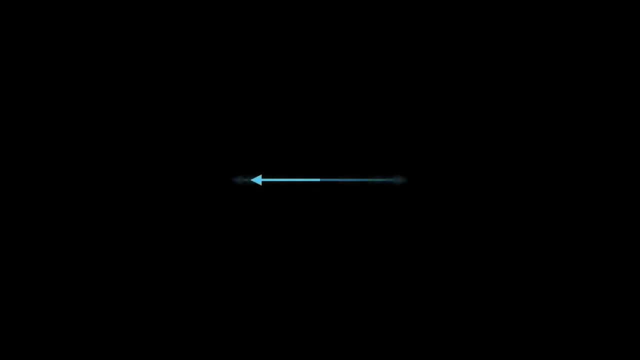 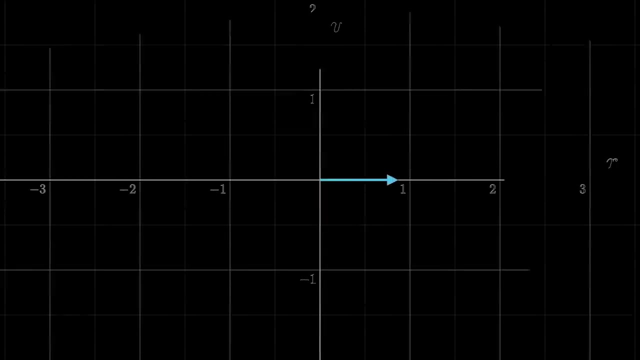 And let's go ahead and ignore the magnetic field right now, just looking at how the electric field oscillates. And also, we're only going to focus on one of these vectors oscillating in the plane of the screen, which we'll think of as the xy-plane. 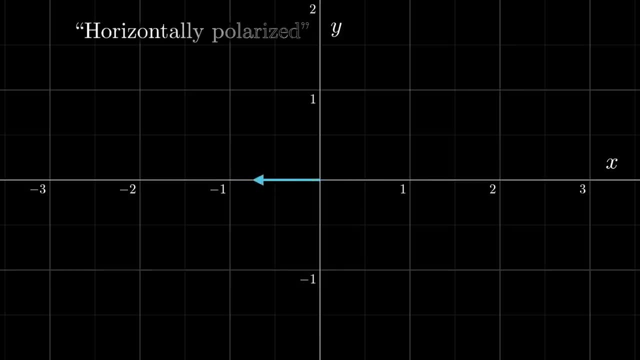 If it oscillates horizontally like this, we say that the light is horizontally polarized. So the y-component of this electric field is zero at all times, and we might write the x-component as something like cos. This is the cosine of 2pi times ft, where f represents some frequency and t is time. 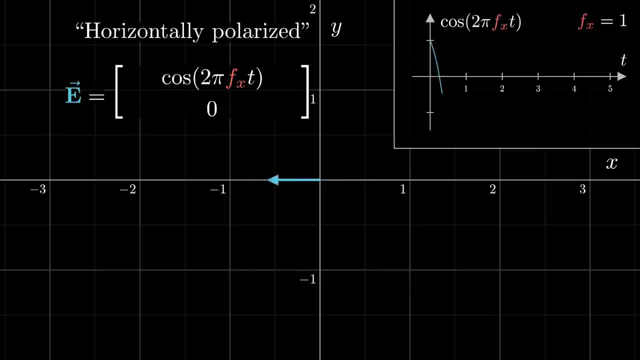 So if f was 1,, for example, that means it takes exactly one second for this cosine function to go through a full cycle. For a lower frequency that would mean it takes more time for the cosine to go through its full cycle. As the value t increases, the inside of this cosine function increases more slowly. 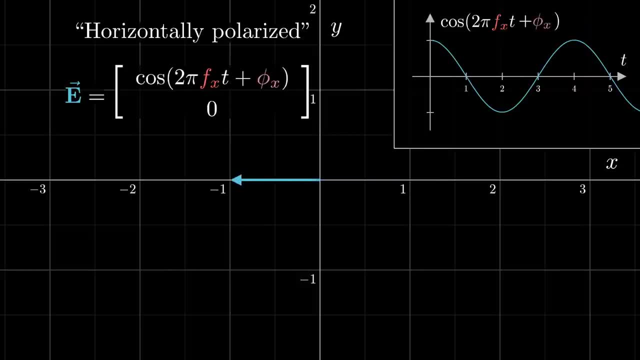 Also, we're going to include another function- Let's put another term in here, phi- called the phase shift, which tells us where this vector is in its cycle. at time t equals zero. You'll see why that matters in just a moment. 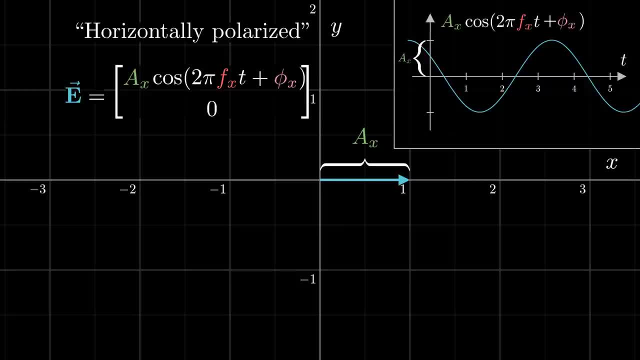 By default, cosine only oscillates between negative 1 and 1.. So let's put another term in front, a, that gives us the amplitude of this wave. One more thing, just to make things look a little more like they often do in quantum. 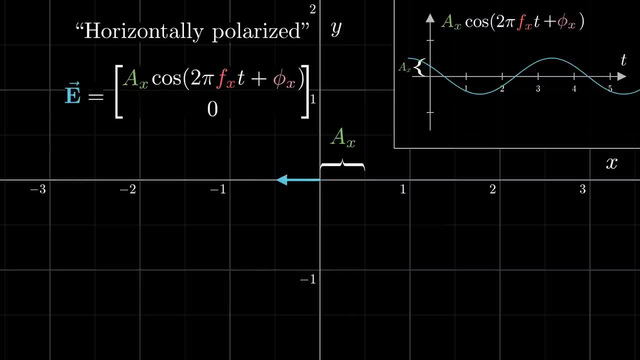 mechanics. Instead of writing it as a column vector like this, I'm going to separate it out into two different components using these symbols called kets. This ket here indicates a unit vector in the horizontal direction, and this ket over here represents a unit vector in the vertical direction. 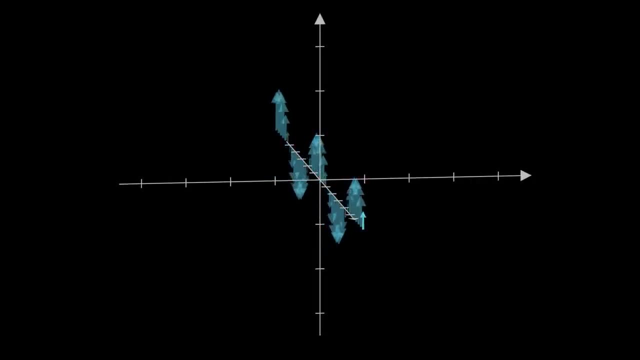 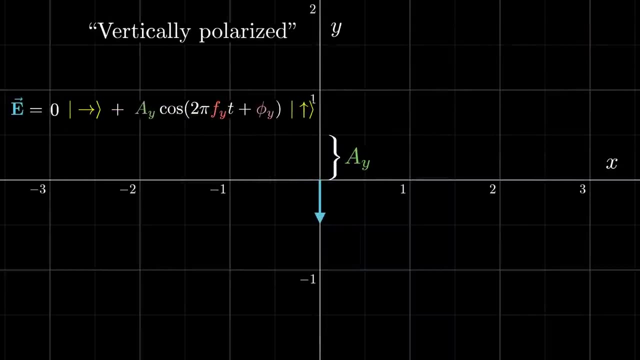 If the light is vertically polarized, meaning the electric field is wiggling purely in the up and down direction, its equation might look like this: where the horizontal component is now zero and the vertical component is a cosine with some frequency, amplitude and 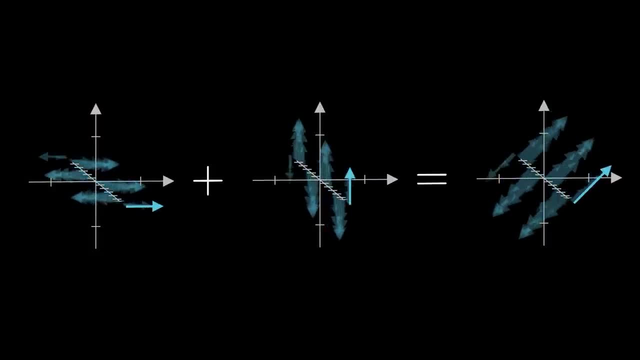 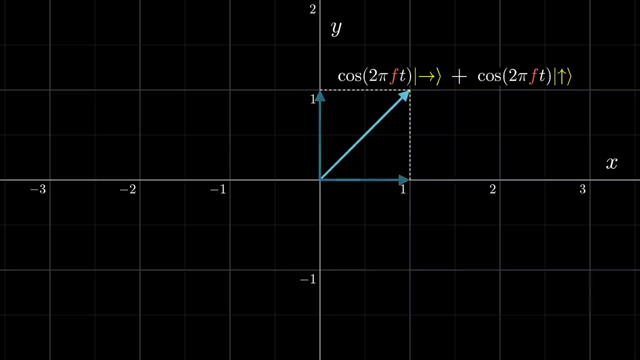 phase shift. Now, if you have two distinct waves, Two waves of wiggling through space over time that solve Maxwell's equations, then adding both of these together gives another valid wave, at least in a vacuum That is at each point in time. add these two vectors tip to tail to get a new vector. 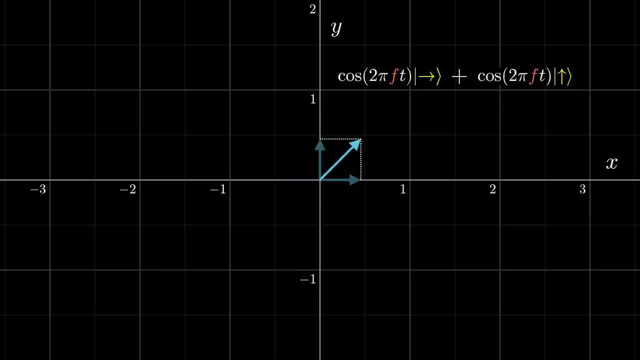 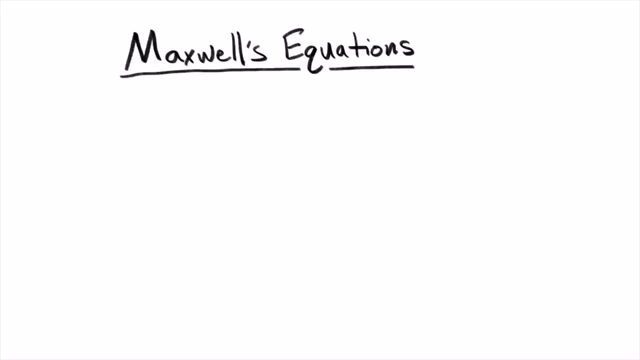 Doing this at all points in space and all points in time gives a new valid solution to Maxwell's equations. At least, this is all true in a vacuum. This is because Maxwell's equations in a vacuum are what's called linear equations. They're essentially a combination of derivatives. 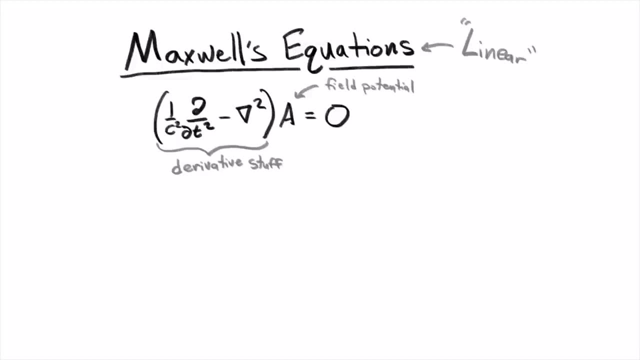 They're derivatives acting on the electric and magnetic fields to give zero. So if one field, F1,, satisfies this equation and another field, F2,, satisfies it, then their sum, F1 plus F2,, also satisfies it, since derivatives are linear. 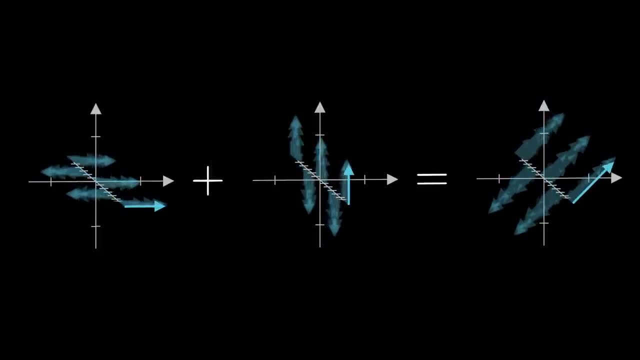 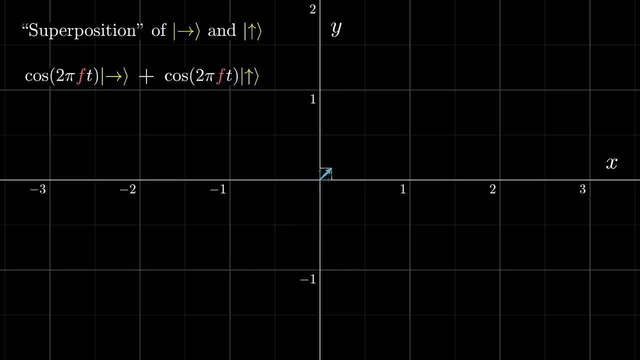 So the sum of two or more solutions to Maxwell's equations is also a solution to Maxwell's equations. This new wave is called a superposition of the first two, And here superposition essentially just means sum, Or in some context weights. 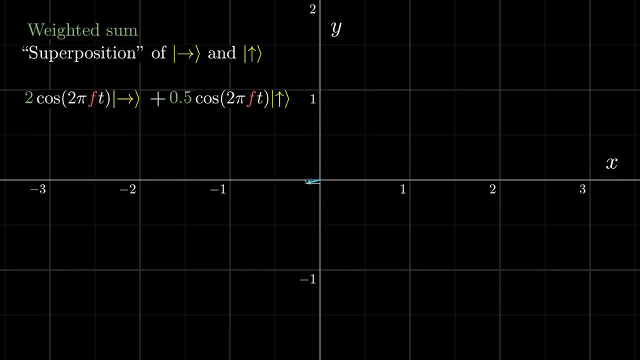 So what does that mean? It's a weighted sum, since if you include some kind of amplitude and phase shift in each of these components, it can still be called a superposition of the two original vectors. Now, right now, the resulting superposition is a wave wiggling in the diagonal direction. 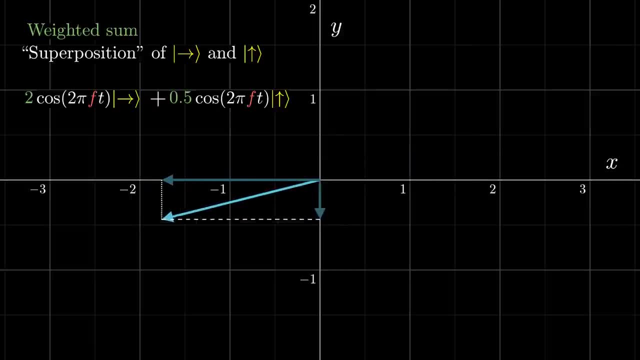 But if the horizontal and vertical components were out of phase with each other, which might happen if you increase the phase shift in one of them, their sum might instead trace out some sort of ellipse. And in the case where the phases are exactly 90 degrees out of sync with each other, and 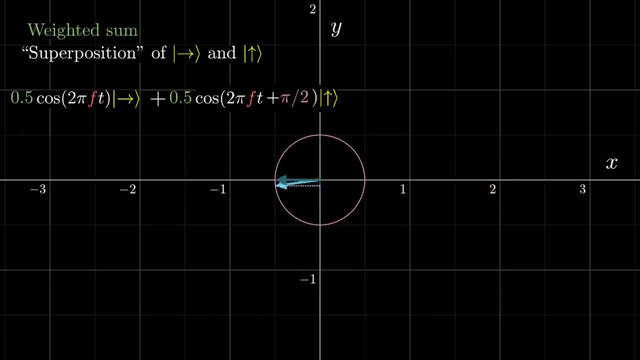 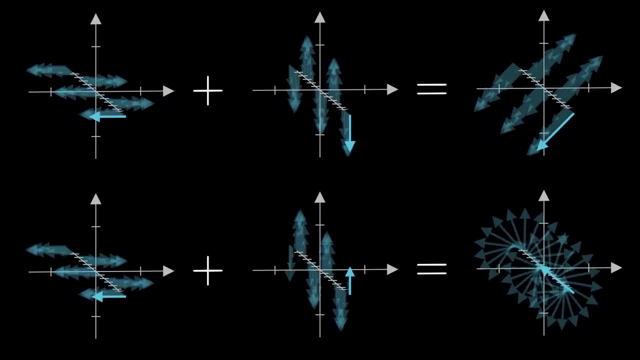 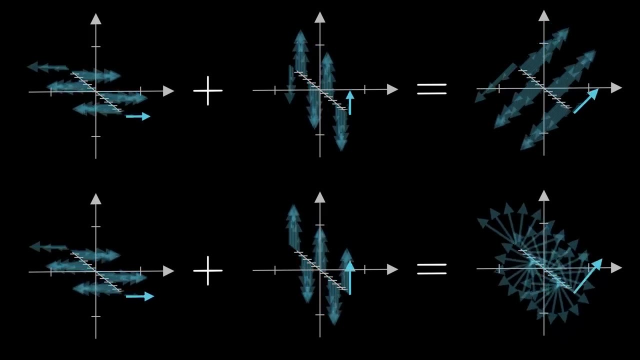 the amplitudes are both equal. this is what we call circularly polarized light. This is why it's important to keep track not just of the amplitude in each direction, but also of the phase It affects the way the two waves add together. 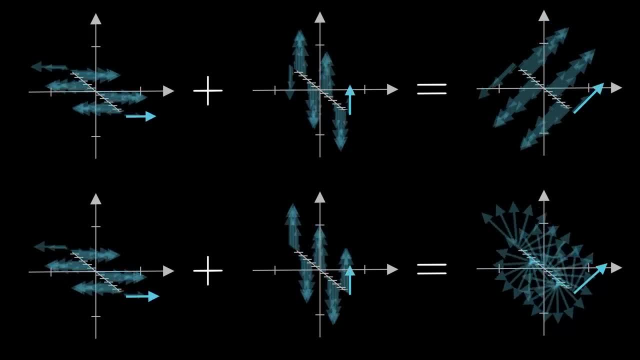 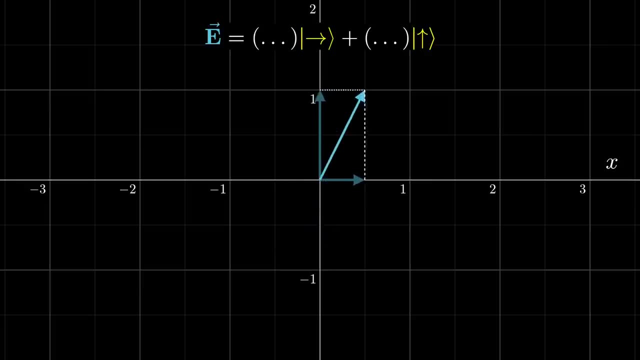 That's also an important idea that carries over to quantum and underlies some of the things that look confusing at first. And here's another important idea: we're describing waves by adding together the horizontal and vertical components, But we could also choose to describe everything with respect to different directions. 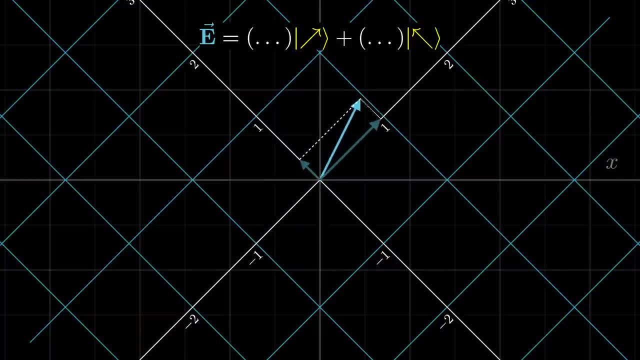 I mean you could describe waves as some superposition of the diagonal and anti-diagonal directions. In that case, vertically polarized light would actually be a superposition of these two diagonal wiggling directions, at least when both are in phase with each other and have the same. 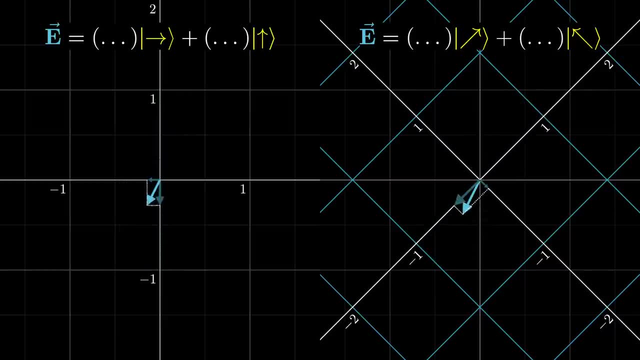 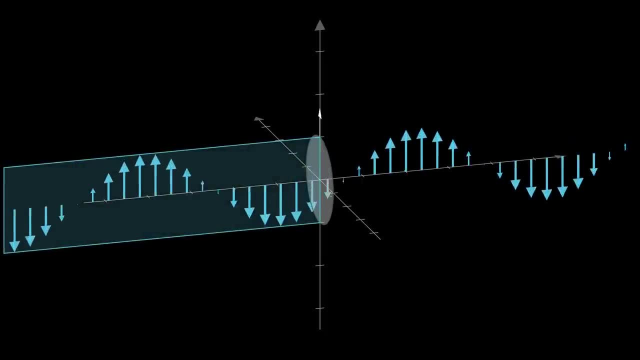 like that, from a set like that, from a set of polarized sunglasses, of polarized sunglasses, of polarized sunglasses. the way these work is, by the way these work is, by the way these work is by absorbing the energy. absorbing the energy, absorbing the energy from electromagnetic oscillations. 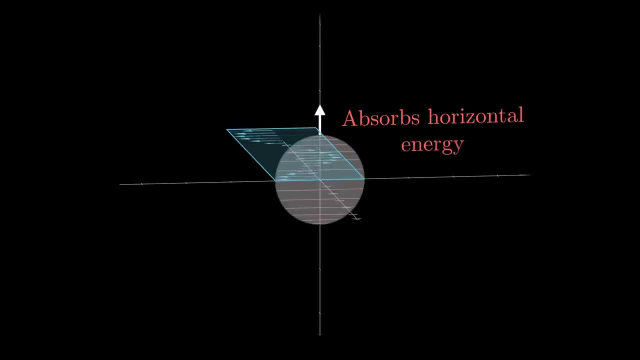 from electromagnetic oscillations, from electromagnetic oscillations in some particular direction, in some particular direction, in some particular direction. A vertically oriented polarizer, A vertically oriented polarizer, A vertically oriented polarizer, for example, would absorb. for example, would absorb. 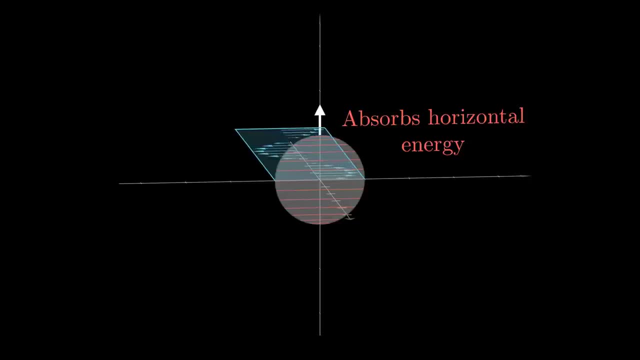 for example, would absorb all of the energy from these waves, all of the energy from these waves, all of the energy from these waves along the horizontal directions, along the horizontal directions, along the horizontal directions, At least classically, At least classically. 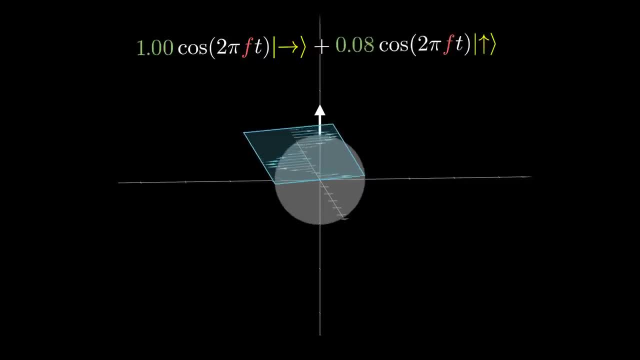 At least classically. that's how you might think, that's how you might think, that's how you might think about it, about it, about it. So, if you're analyzing light, So if you're analyzing light, So if you're analyzing light and it's passing through, 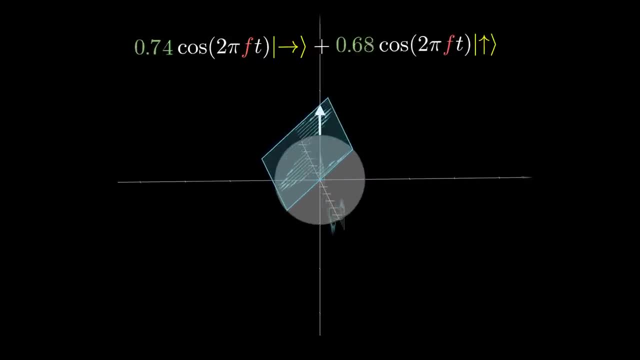 and it's passing through. and it's passing through a filter like this, a filter like this, a filter like this, it's nice to describe it, it's nice to describe it, it's nice to describe it with respect to the horizontal, with respect to the horizontal. 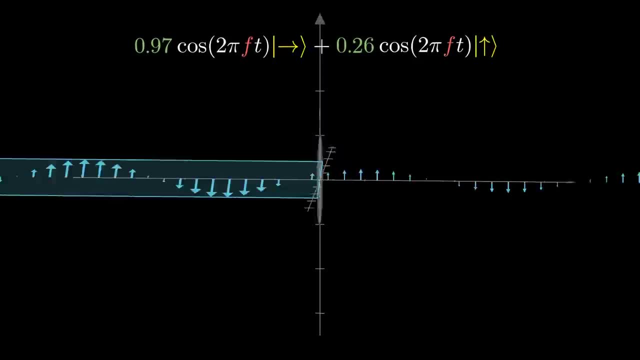 with respect to the horizontal and vertical directions, and vertical directions and vertical directions. That way, what you can say That way, what you can say That way, what you can say is that whatever light is that, whatever light is that, whatever light passes through the filter. 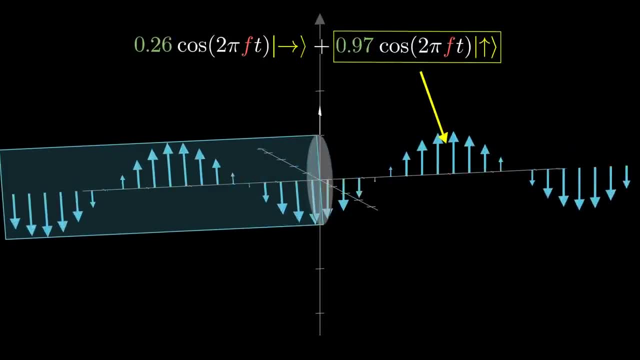 passes through the filter, passes through. the filter is just the vertical component, is just the vertical component, is just the vertical component of the original wave, of the original wave, of the original wave. But if you had a filter oriented, But if you had a filter oriented, 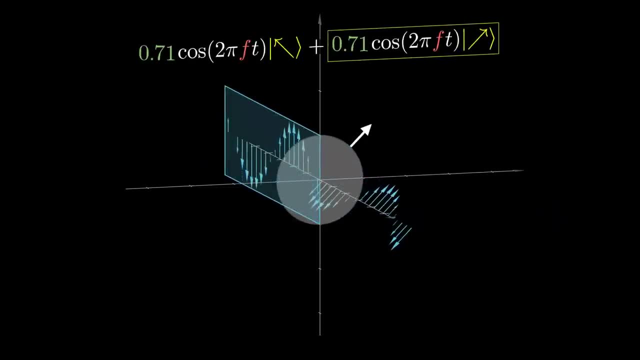 But if you had a filter oriented, say diagonally well, say diagonally well, say diagonally well, then it would be convenient, then it would be convenient, then it would be convenient to describe things as a, to describe things as a. 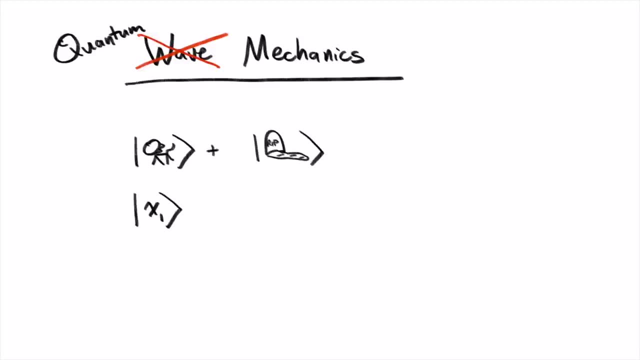 to describe things as a superposition case, superposition case, superposition case, Quantum states. much like this Quantum states. much like this Quantum states, much like this wiggling direction of our wave, wiggling direction of our wave. 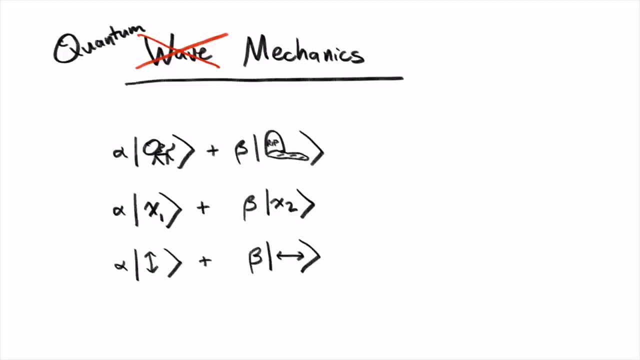 wiggling direction of our wave are described as a superposition, are described as a superposition, are described as a superposition of multiple base states, of multiple base states, of multiple base states, where you have many choices, where you have many choices. 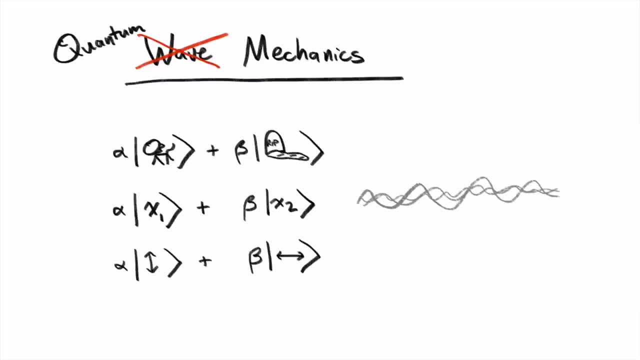 where you have many choices for what base states to use, for what base states to use, for what base states to use, And just like with classical, And just like with classical, And just like with classical waves, the components of such waves, the components of such. 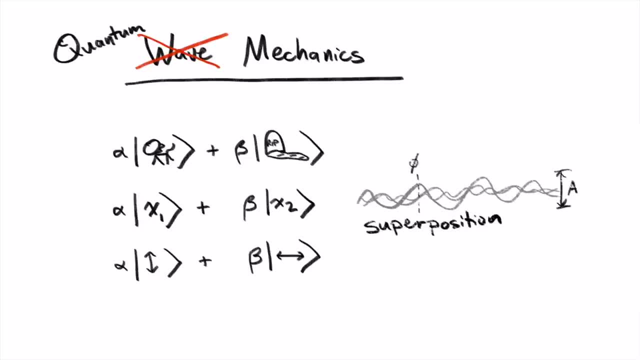 waves. the components of such a superposition will have a superposition will have a superposition will have both an amplitude. a superposition will have both an amplitude. a superposition will have both an amplitude and a phase of some kind and a phase of some kind. and a phase of some kind. And, by the way, for those of you, And by the way for those of you, And by the way, for those of you who do read more into quantum, who do read more into quantum, who do read more into quantum mechanics, you'll find that 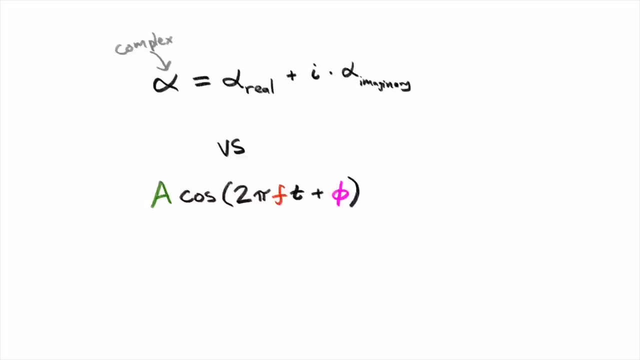 mechanics, you'll find that. mechanics, you'll find that these components are actually. these components are actually. these components are actually given using a single complex. given using a single complex. given using a single complex number rather than a cosine number, rather than a cosine number rather than a cosine expression like this one. 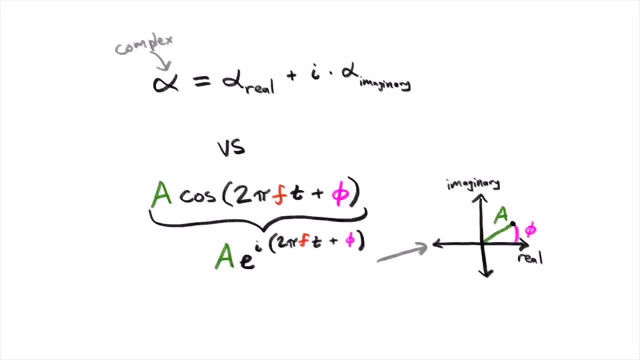 expression like this one, expression like this one. One way to think of this is that One way to think of this is that complex numbers are just a very convenient and natural mathematical way to encode an amplitude and a phase with a single value. That can make things a. 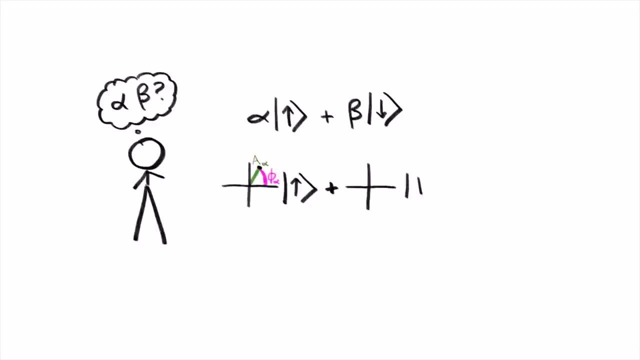 little confusing, because it's hard to visualize a pair of complex numbers, which is what would describe a superposition of two base states. But you can think about the use of complex numbers throughout quantum mechanics, as a result of its underlying wavy nature and this need to encapsulate the 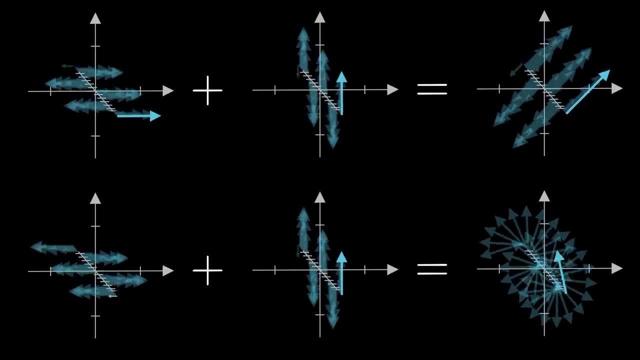 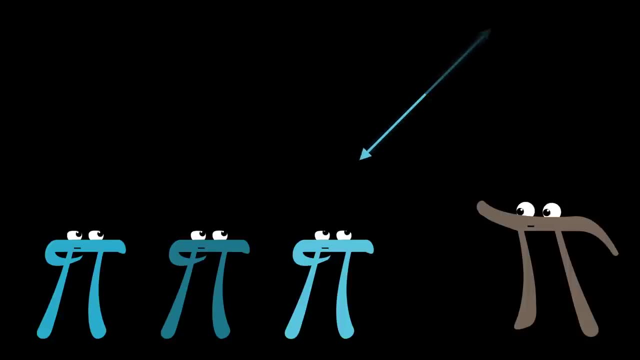 amplitude and the phase for each direction. Okay, just one quick point before getting into the quantum. Look at one of these waves and focus just on the electric field portion, like we were before. Classically, we think about the energy of a wave like this as being proportional to the square of its 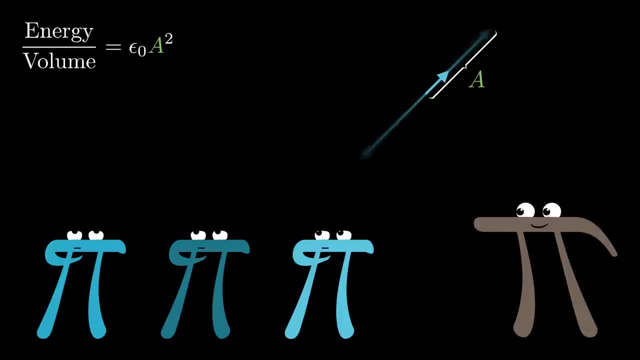 amplitude, and I want you to notice how well this lines up with the Pythagorean theorem. If you were to describe this wave as a superposition of a horizontal component with amplitude AX and a vertical component with amplitude AY, then its energy density is proportional to AX squared plus AY squared, And you 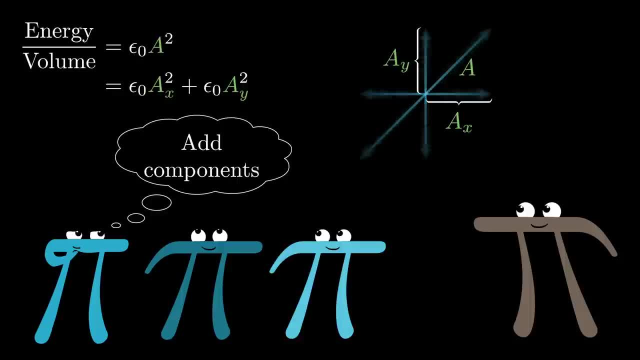 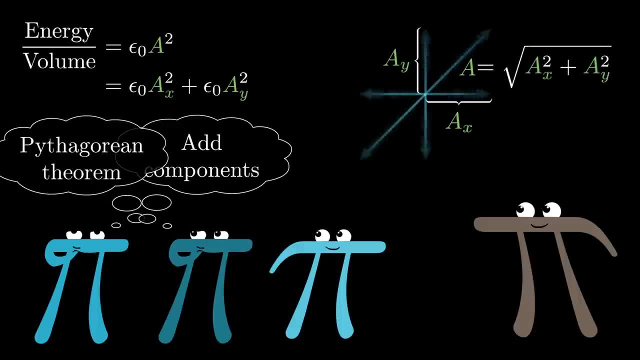 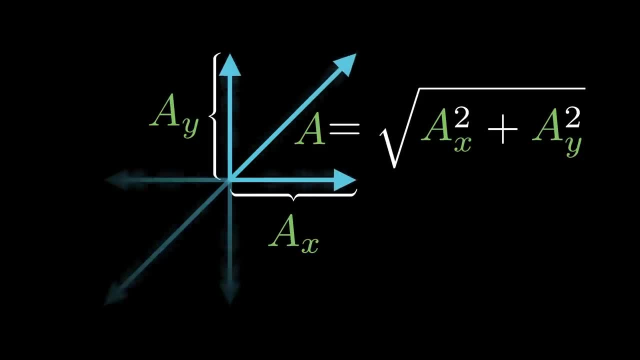 superposition, or it's just that you're figuring out the new amplitude using the Pythagorean theorem and taking the square. Isn't that nice? In the classical understanding of light, you should be able to dial this energy up and down continuously however you want, by changing the amplitude of the wave. But 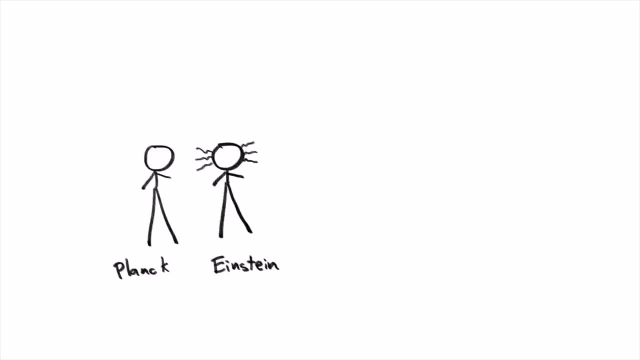 what physicists started to notice in the late 19th and early 20th centuries was that this energy actually seems to come in discrete amounts. Specifically, the energy of one of these electromagnetic waves always seems to come as an integer multiple of a specific constant times. the frequency of 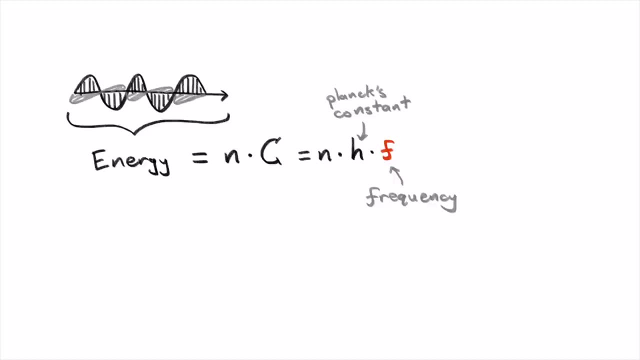 that wave. We now call this constant Planck's constant, commonly denoting it with the letter h. Physically, what this means is that whenever this wave trades its energy with something else, like an electron, the amount of energy it trades off is always an integer multiple of h times its 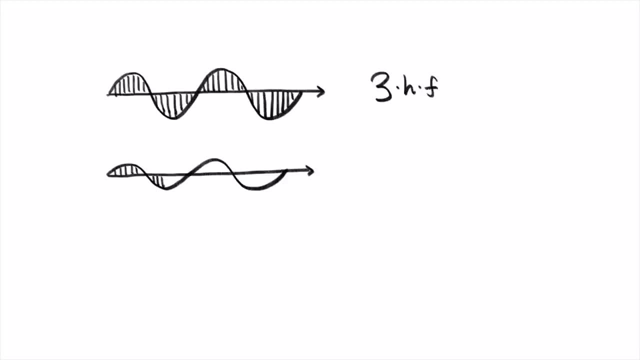 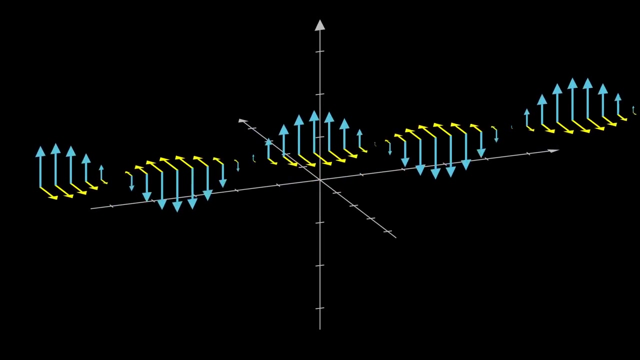 frequency. Importantly, this means there is some minimal, non-zero energy level for waves of a given frequency, hf. If you have an electromagnetic wave with this frequency and energy, you cannot make it smaller without eliminating it entirely. That feels weird when the conception of a wave is a nice, continuously oscillating vector field. 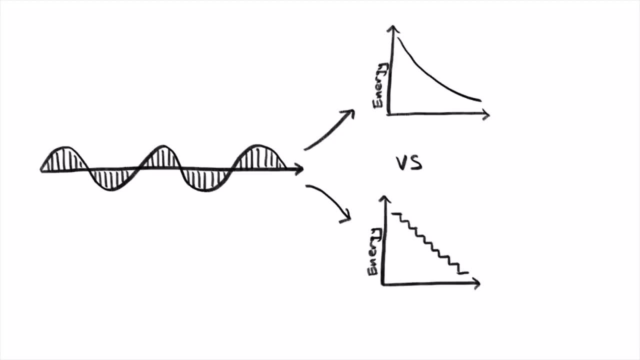 but that's not how the universe works, as late 19th and early 20th century experiments started to expose. In fact, I've done a video about this, called the Origin of Quantum Mechanics. However, it's worth noting that this phenomenon is 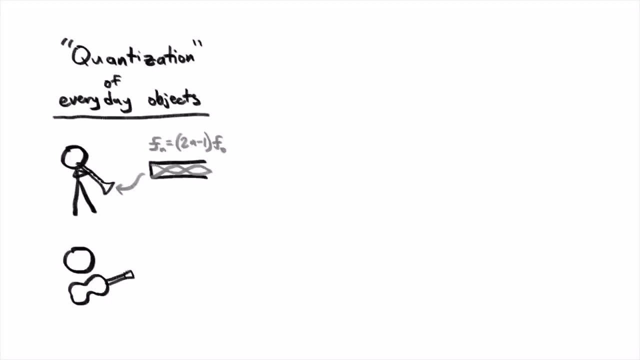 actually common in waves when they're constrained in certain ways, like in pipes or instrument strings, and it's called harmonics. What's weird is that electromagnetic waves do this in free space. and that's because the waves are free space even when they're not constrained. And what do we call an electromagnetic wave with? 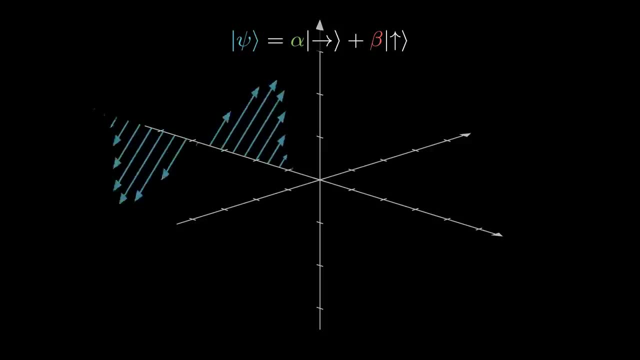 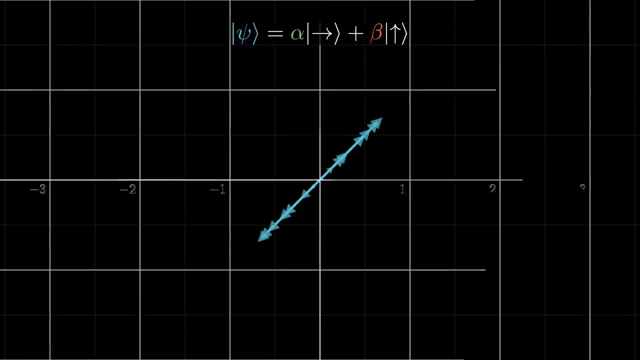 this minimal possible energy, A photon. But like I said, the math used to describe classical electromagnetic waves carries over to describing a photon. It might have, say, a 45 degree diagonal polarization which can be described as a superposition of a purely 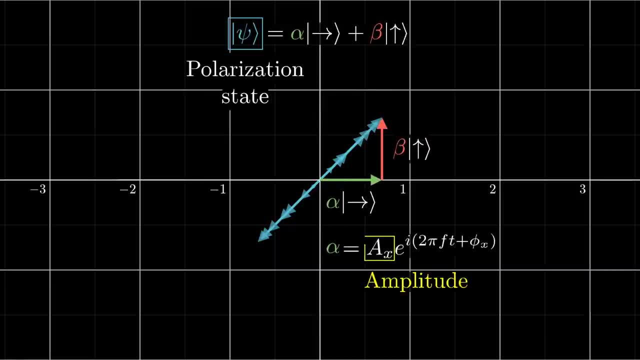 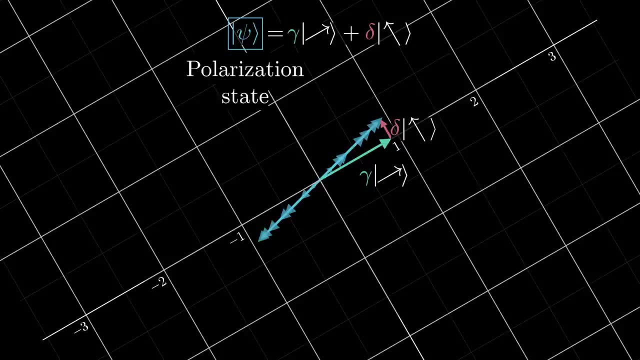 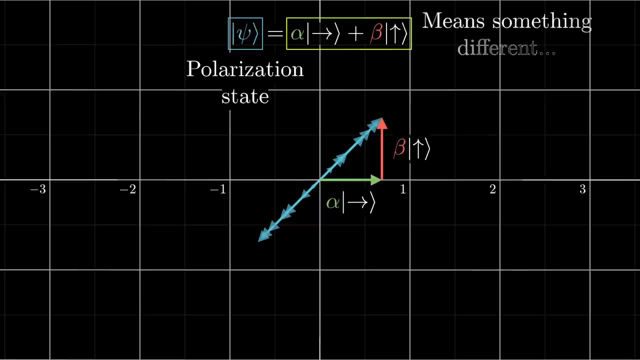 horizontal state and a purely vertical state, where each one of these components has some amplitude and phase And with a different choice in bases. that same state might be described as a superposition of two other directions. All of this is stuff that you would see if you started reading more into quantum mechanics, But this superposition has a different. 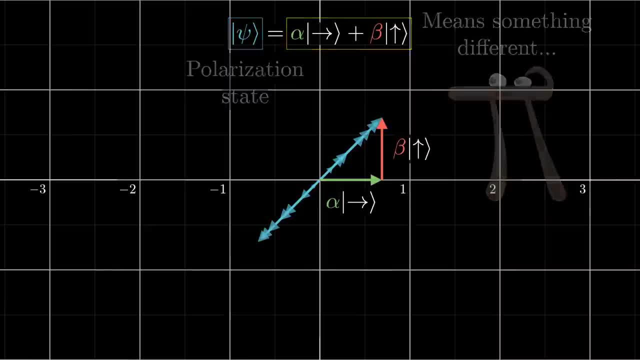 interpretation than before, and it has to. Let's say, you were thinking of this diagonally polarized photon kind of classically and you said it has an amplitude of one unit for some appropriate unit system. Well, that would make the hypothetical amplitudes of its horizontal and vertical. 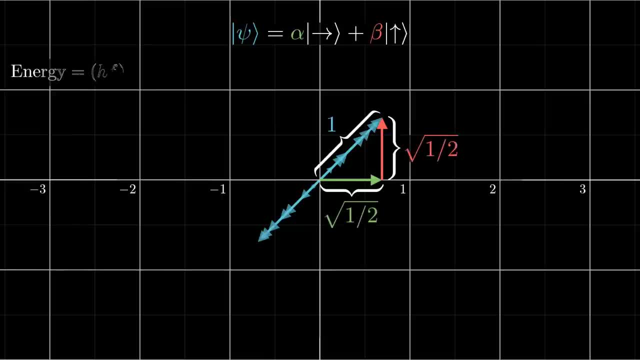 components, each the square root of one half. And, like Henry said, the energy of a photon is this special constant: h times its frequency. And because, in a classical setting, energy is proportional to the square of the amplitude of this wave, it's tempting to think. 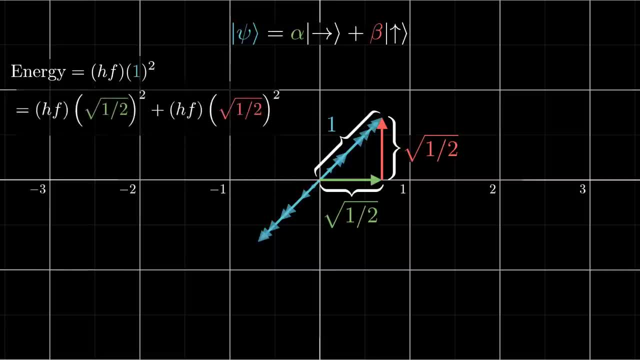 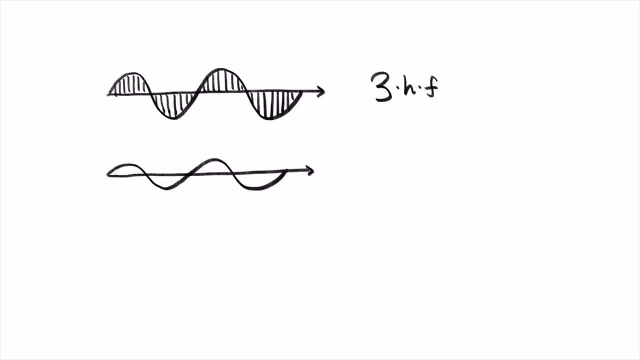 of half of the energy as being in the horizontal component and half of it as being in the vertical component. But waves of this frequency cannot have half the energy of a photon. I mean, the whole novelty of quantum here is that energy comes in these discrete, indivisible chunks. So 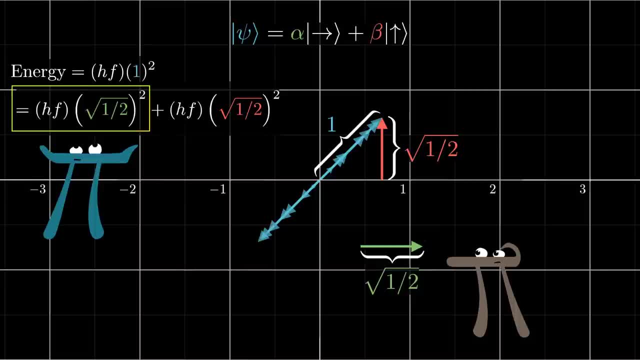 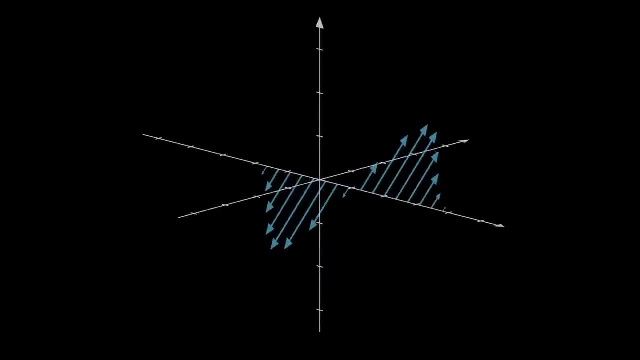 these components, with an imagined amplitude of 1 over the square root of one half, are not in isolation, And you might wonder what exactly they mean. Well, let's get experimental about it. If you were to take a vertically oriented polarizing, 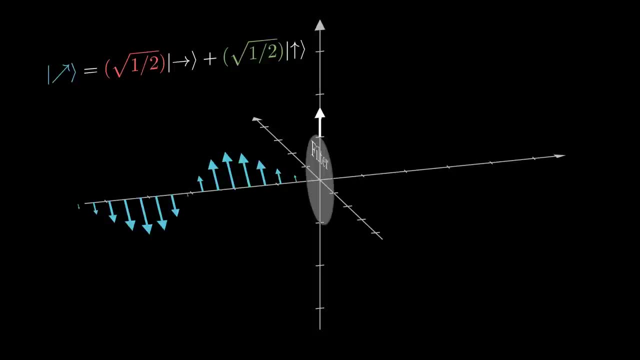 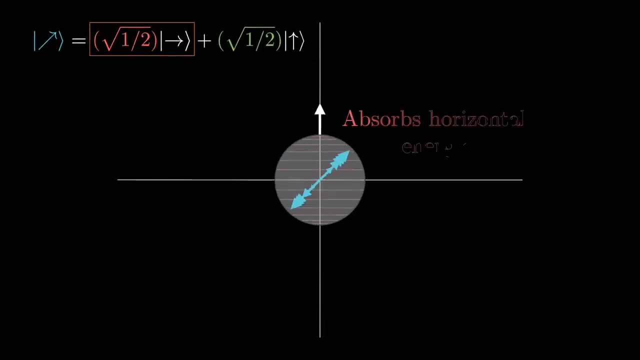 filter and shoot this diagonally polarized photon right at it. what do you think would happen? Classically, the way you'd interpret this superposition is that the half of its energy in the horizontal direction would be absorbed. But because energy comes in these discrete photon, 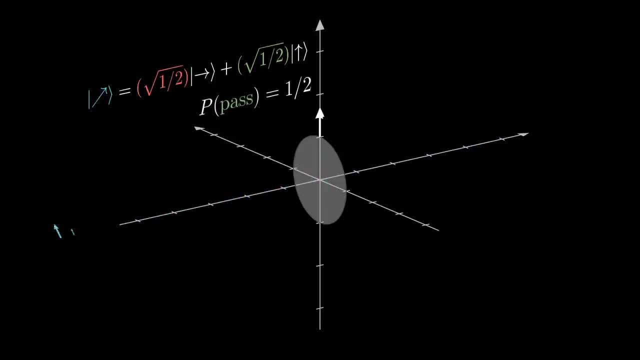 packets. it either has to be in the horizontal component or it has to be in the horizontal component. And that's exactly what we're going to do here. We're going to use this superposition to pass through with all its energy or get absorbed entirely. And if you actually did this, 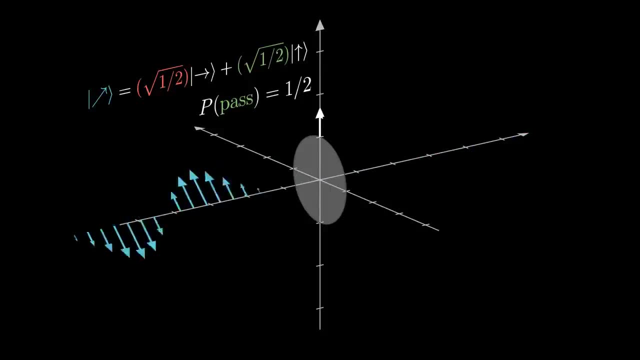 experiment. about half the time the photon goes through entirely and about half the time it gets absorbed entirely, And it appears to be random whether a given photon passes through or not. If it does pass through, forcing it to make a decision like this actually changes it. so 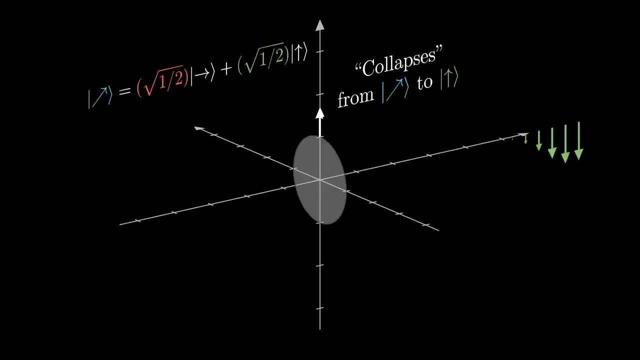 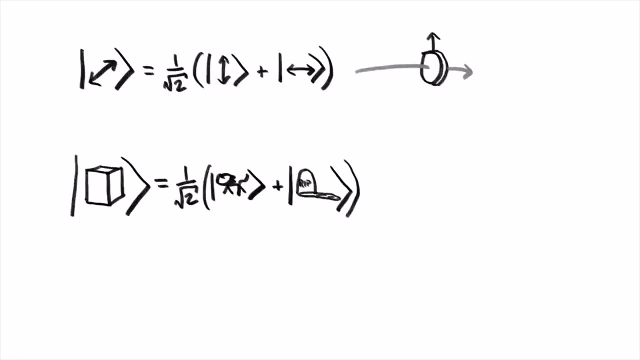 that its polarization is oriented along the filter's direction. This is analogous to the classic Schrodinger's cat setup. You have something that's in a superposition and you can make a superposition of two states, but once you make a measurement of that superposition, 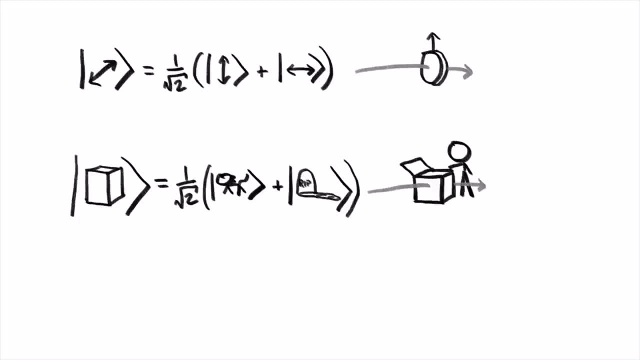 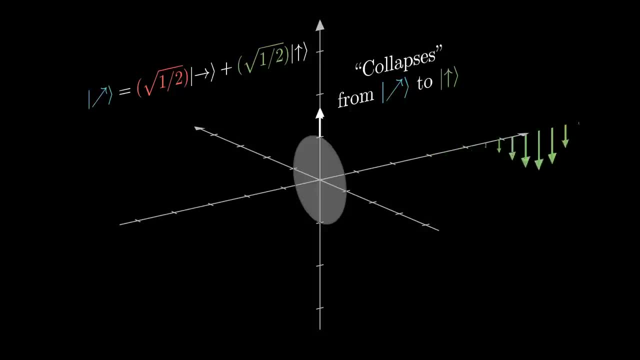 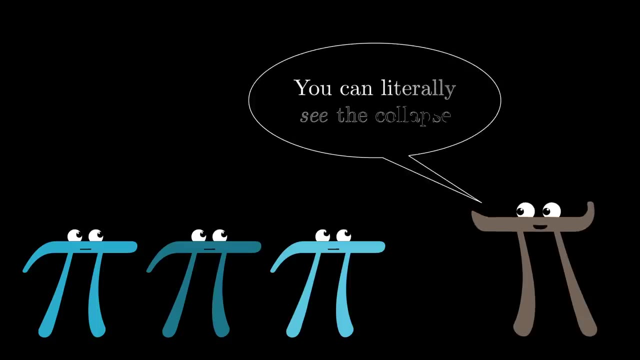 forcing it to interact with an observer in a way where each of those two states would behave differently. from the perspective of that observer, this superposition collapses to be entirely in one state or entirely in another, dead or alive, horizontal or vertical. One pretty neat way to see this in action, which Henry and I talk about in the other video. 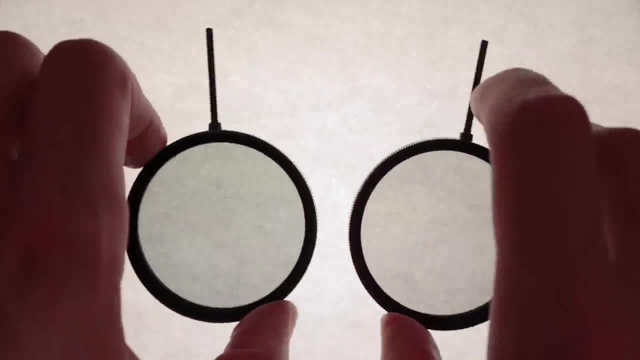 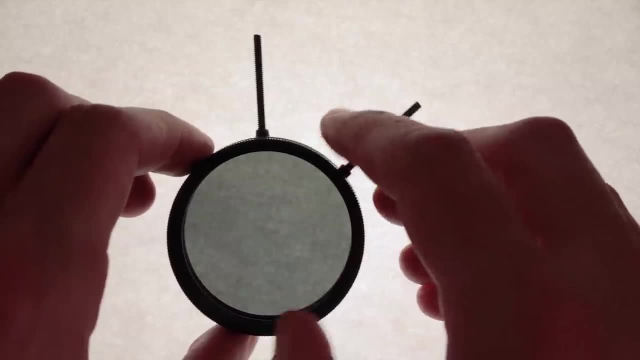 is to take several polarized sunglasses or some other form of polarizing filters and start by holding two of them between you and some light source. If you rotate them to be 90 degrees off from each other, the light source is blacked out completely, or at least with perfect. 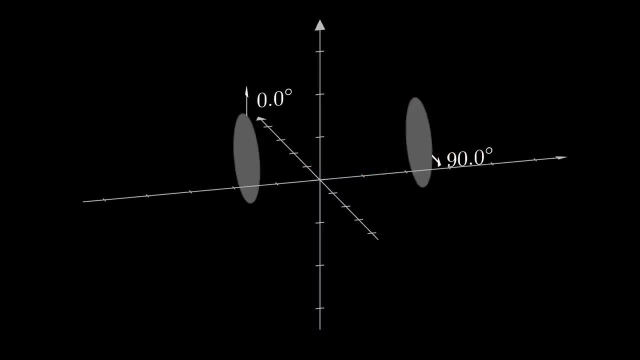 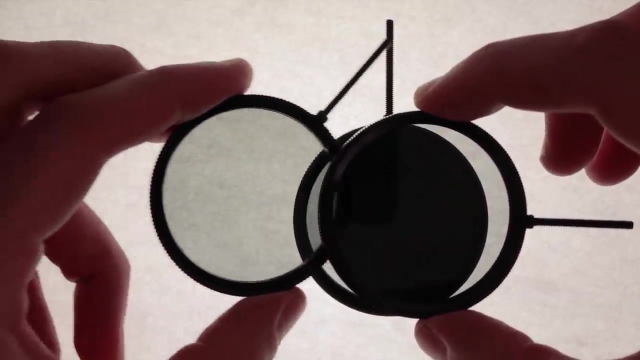 filters. it would be Because all of the photons passing through that first one are polarized vertically, so they actually have a 0% chance of passing a filter oriented horizontally. But if you insert a third filter oriented at a 45 degree angle between the two, it actually lets. 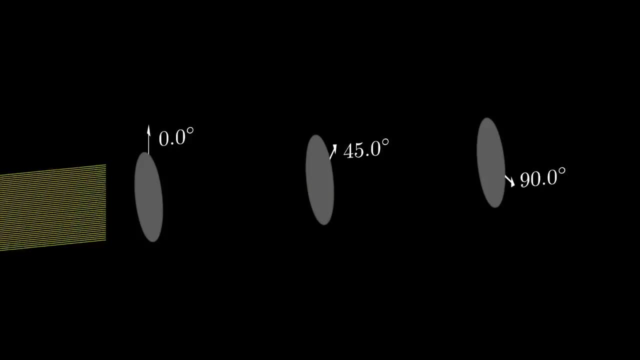 more light through. And what's going on here is that 50% of the photons passing that vertical filter will also pass through the diagonal filter And once they do, they're going to be changed to have a purely diagonal polarization And then, once they're in that state, they have a 50-50 chance of passing through the. 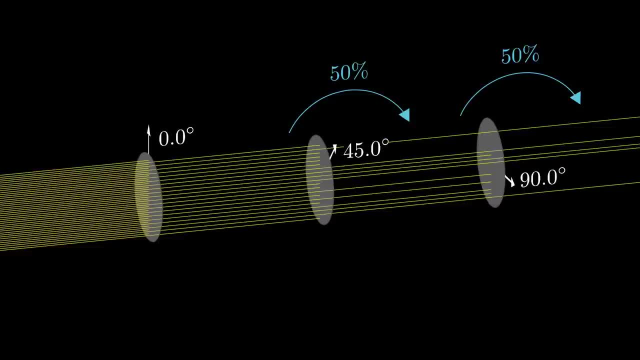 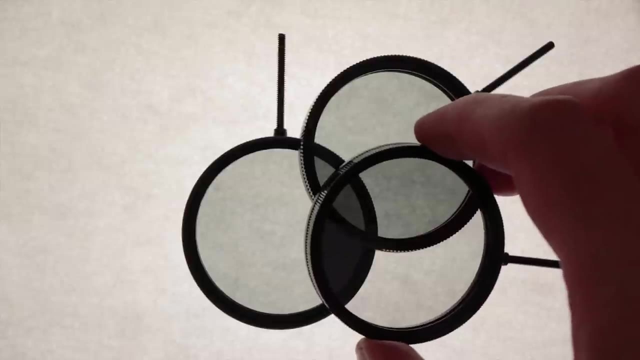 filter oriented at 90 degrees. So even though 0% of the photons passing through the first would pass through that last if nothing was in between, by introducing another filter, 25% of them now pass through all three. Now that's something that you could not explain, unless that middle filter forces the photons. 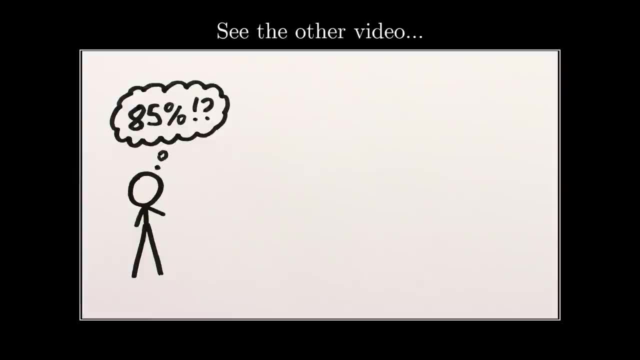 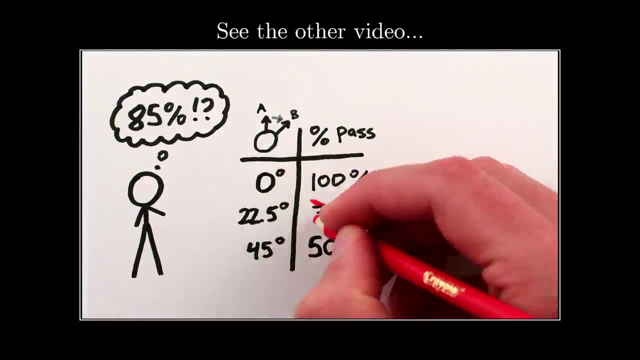 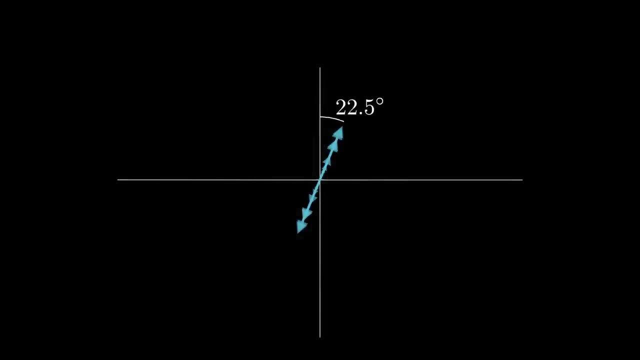 to change their states. And that experiment, by the way, becomes all the weirder when you dig into the specific probabilities for angles between 0 and 45 degrees, And that's actually what we talk about in the other video. For example, one specific value we focus on there is the probability that a photon whose 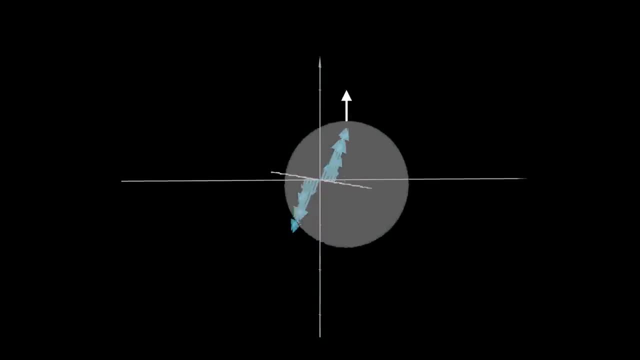 polarization is 22.5 degrees off, the direction of a filter is going to end up passing through that filter. Again, it's helpful to think of this wave as having an amplitude of 1, and then you'd think of the horizontal component as having amplitude sine of 22.5 degrees, which is around. 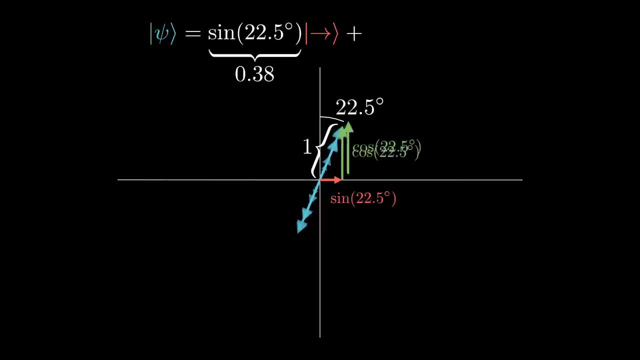 0.38, and the vertical component would have an amplitude cosine of 22.5 degrees, which is around 0.92.. Classically, you might think of its horizontal component as having energy proportional to 0.38 squared, which is around 0.92.. 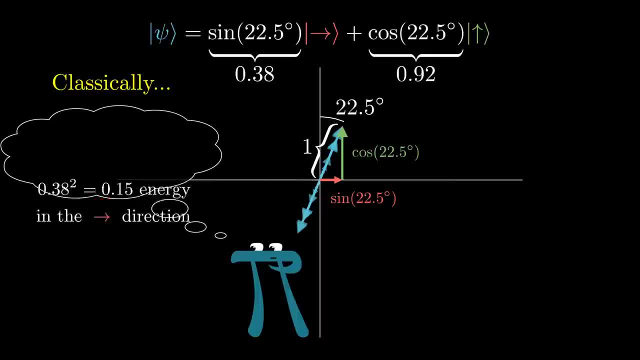 Likewise, you might think of the vertical component as having an energy proportional to 0.92 squared, which comes out to be around 0.85.. And, like we said before, classically this would mean, if you pass it through, a vertical 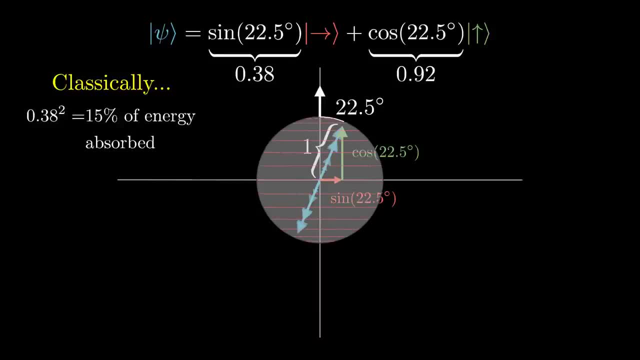 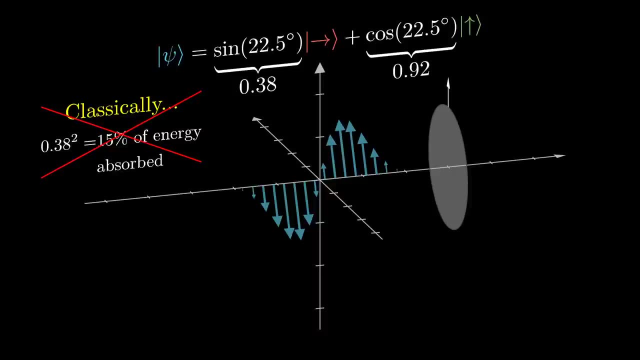 filter. 15% of its energy is absorbed in the horizontal direction, But because the energy of light comes in these discrete quanta that cannot be subdivided. instead, what you observe is that 85% of the time, the photon passes through entirely. 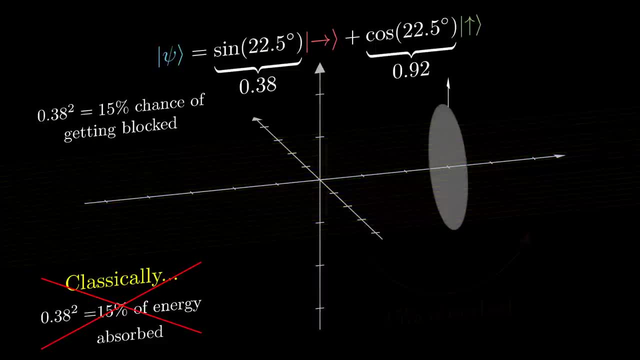 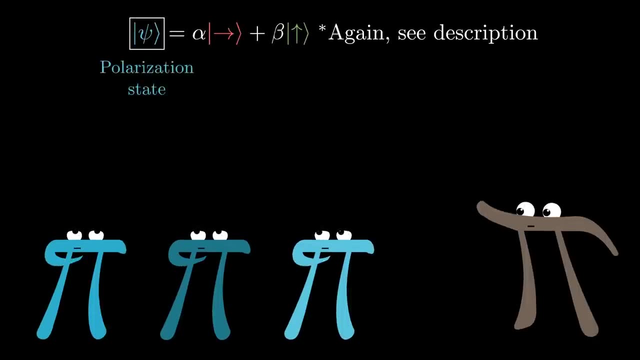 and 15% of the time it gets completely blocked. Now I want to emphasize that the wave equations don't change. The photon is still described as a superposition of two oscillating components, each with some phase and amplitude, and these are often encoded using a single complex number. 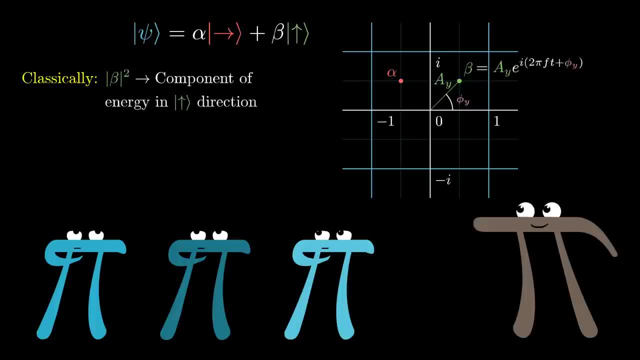 The difference is that, classically, the squares of the amplitudes of each component tells you the amount of that wave's energy in each direction. But with quantized light, At this minimal, non-zero energy level, the squares of those amplitudes tell you the probabilities. that a given photon is going to be found to have all of its energy in one direction or not. Also, these components could still have some kind of phase difference. Just like with classical waves, photons can be circularly polarized and there exist polarizing. 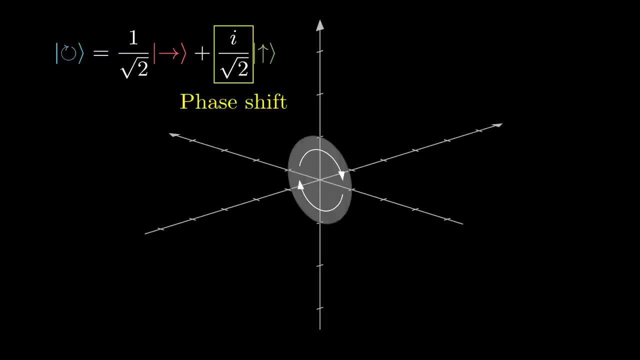 filters that only let through photons that are polarized circularly, say in the clockwise direction, Or rather, they let through all photons probabilistically. This is what we call a phase difference, Where the probabilities are determined by describing each one of those photons as a 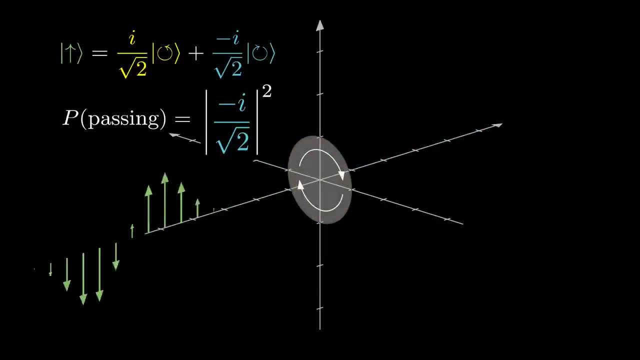 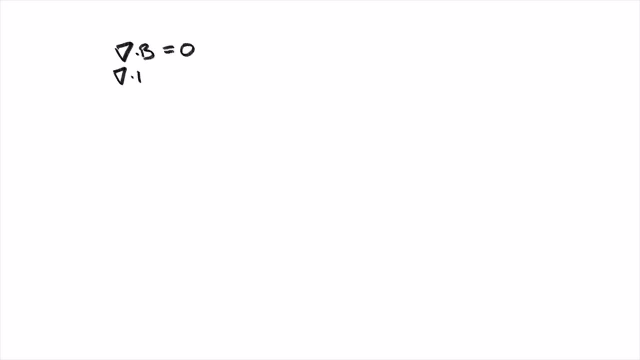 superposition of the clockwise and counterclockwise states, and then the square of the amplitude of the clockwise component gives you the desired probability. Photons are, of course, just one quantum phenomenon, one where we initially understood it as a wave, thanks to Maxwell's equations, and then as individual particles or quanta. hence the 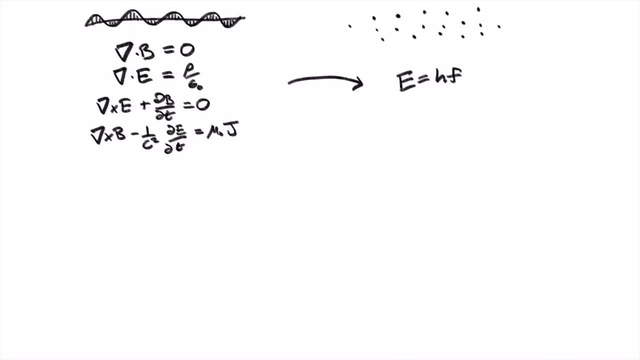 name quantum mechanics, But, as many of you well know, there's a flipside to this, where many things that were understood to come indiscreetly don't. Little packets like electrons, were discovered to be governed by similar wavy quantum mechanics. 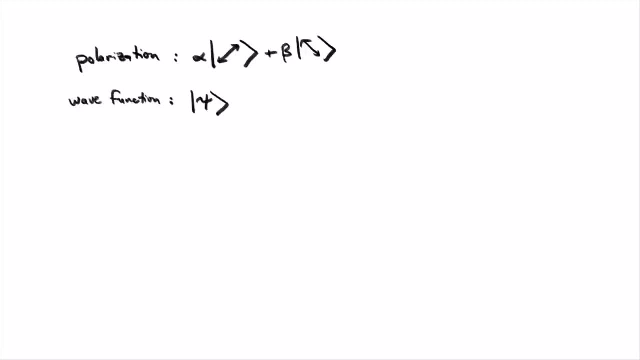 In cases way more general than this- one photon polarization example. quantum mechanical states are described as some superposition of multiple base states, and the superposition depends on what basis you choose. Each component in this superposition is given with an amplitude and a phase, often encoded. 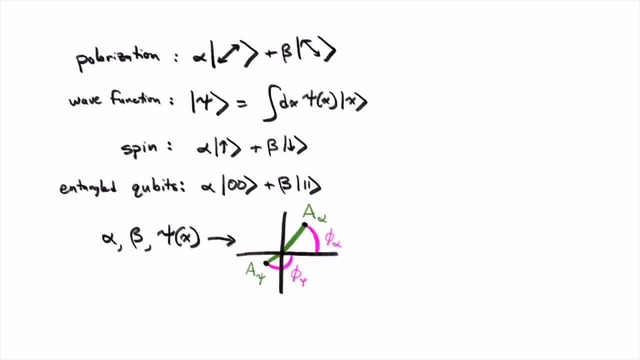 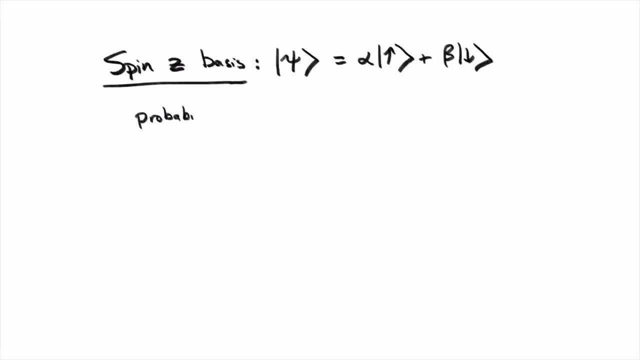 as a single complex number, and the need for this phase arises from the wave nature of these objects. As with the photon example, the choice of how to measure these objects can determine a set of base states, where the probability of measuring a particle to be in one of these